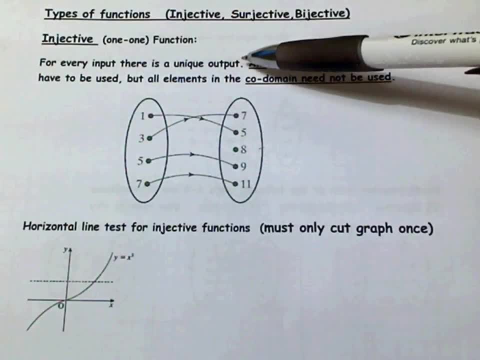 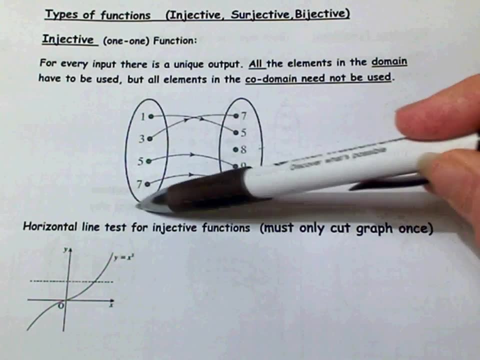 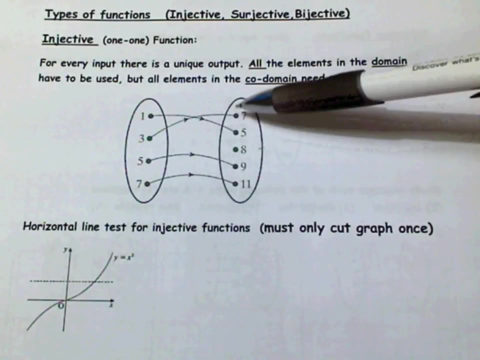 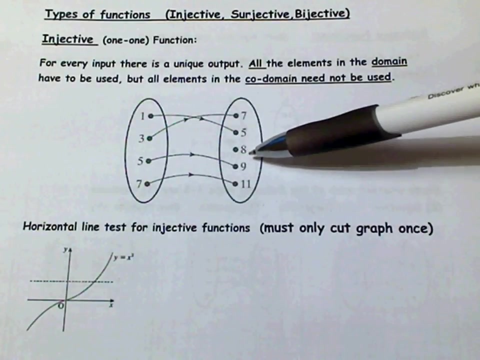 And so for every input there is a unique output. That is very important. All the elements in the domain have been used. So here's our domain, or our input values, And all the elements in the domain have to be used in an injective function. But all the elements in the co-domain do not have to be used. So you can see here that eight is not used. But this is an injective function because all of the inputs have unique outputs. One goes to five. 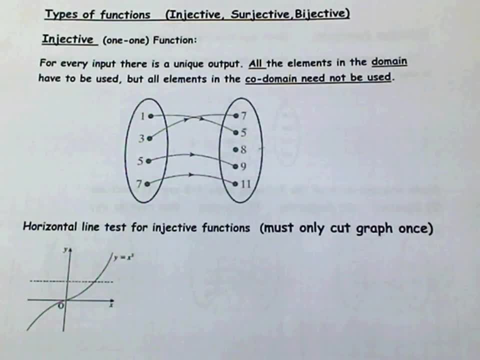 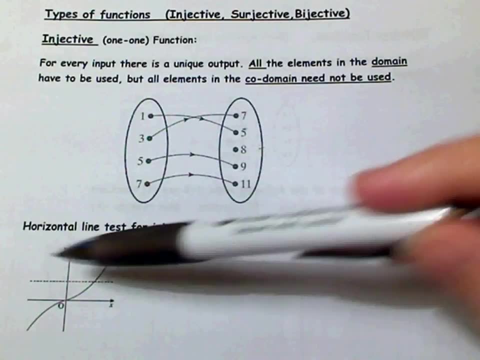 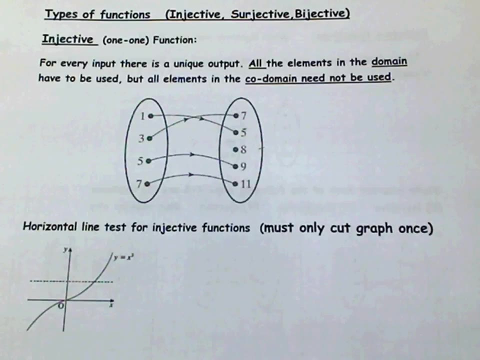 three goes to seven, five goes to nine and seven goes to eleven. Now, if you look down also, a test for an injective function is if you draw a horizontal line across through the graph. For an injective function, the horizontal line can only cut the graph once. 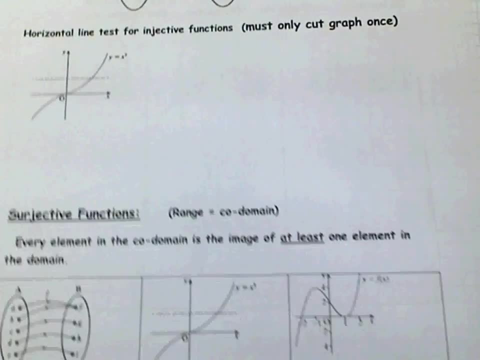 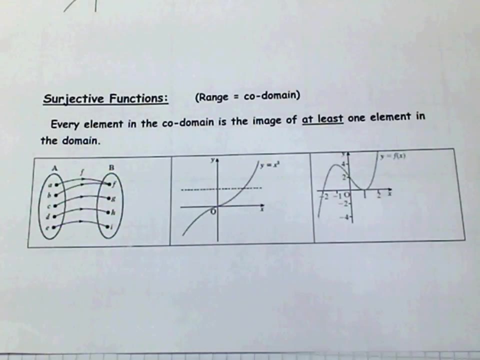 Now the next type of function is a surjective function. Okay, so for a surjective function, every element in the co-domain- so here's our co-domain over here- is the image of at least one element in the domain. Okay, so look at the difference between it and the injective function. This is a surjective function. A goes to F, but B can also go to F. They don't exactly have to have unique outputs. C goes to G, D goes to H and E goes to I. Now, all of the co-domain have to be used in an injective function. So here's our co-domain over here: Every element in the co-domain- so here's our co-domain over here- is the image of at least one element in the domain. Okay, so look at the difference between it and the injective function. This is a surjective function. A goes to F, but B can also go to F. They don't exactly have to have unique outputs. C goes to G, D goes to H and E goes to I. Now, all of the 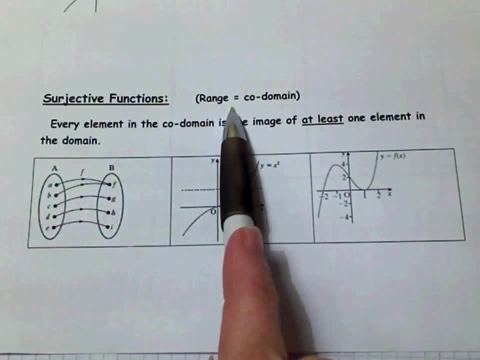 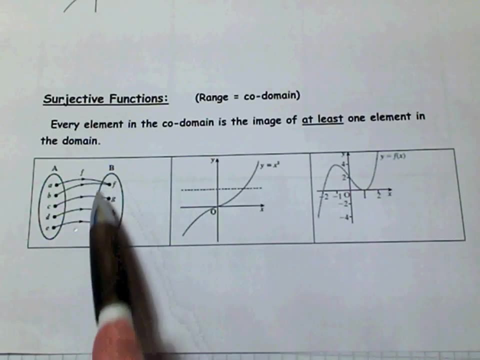 has been used. so this is very important. in a surjective function, the range is equal to the codomain, because every single value in the codomain has been used in the range. every single input and, as used up, all of the possible outputs are all of the part, all of the elements in the codomain. now for a surjective. 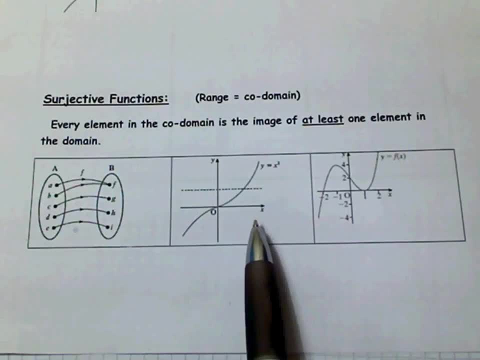 function and you use the horizontal line test again. now both of these graphs are surjective functions. this is a surjective function because the horizontal line cuts the graph at least once. okay, now I know that I said for an injective function it could only cut it once, but this cuts it at least. 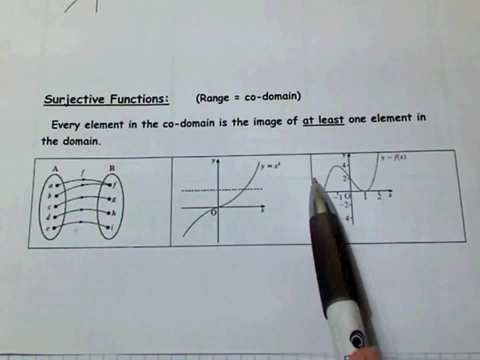 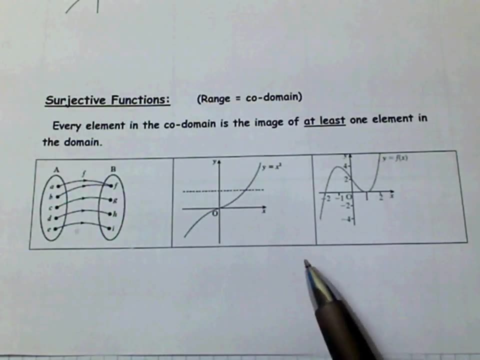 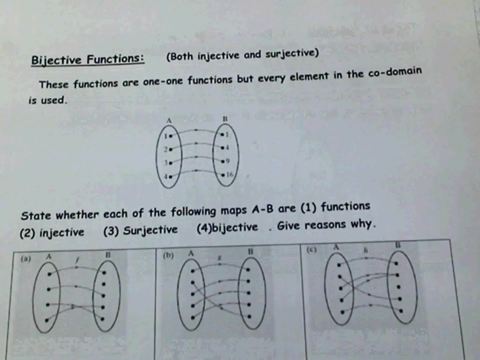 once. this is also a surjective function, because the horizontal line cuts it at least once and you can see there, it'll cut it once, twice, three times in this particular function. now moving on to our next type of functions, which are bijective functions. okay, now a bijective function. 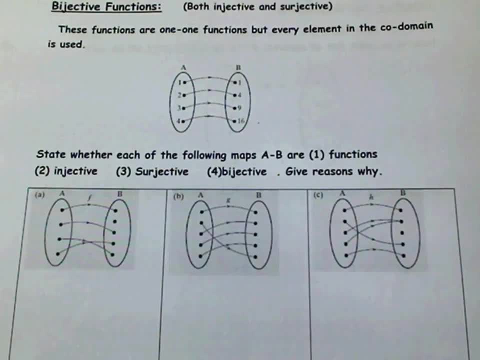 is a function which is both injective and surjective. okay, these functions are one to one function, but every element in the codomain is used. okay, so remember, one of the conditions for a surjective function was every element in the codomain used. okay, so a bijective function if asked to. 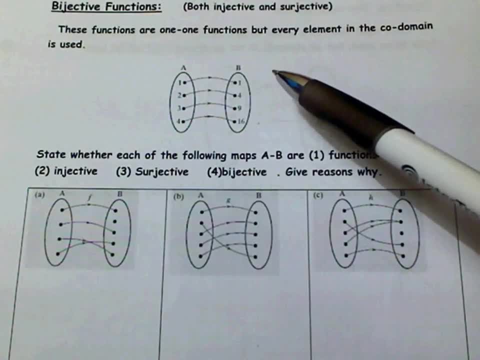 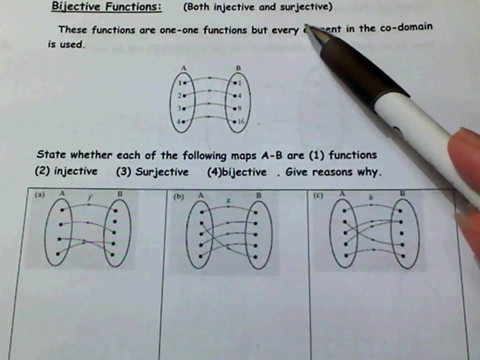 describe a function and say if it's bijective, look to see if it's both injective and surjective, and what's very important with surjective is also to make sure that the range is equal to the codomain. now it's a very good example. 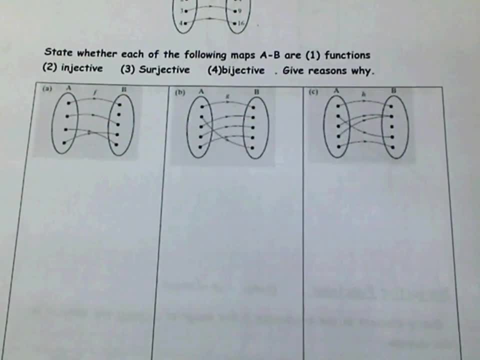 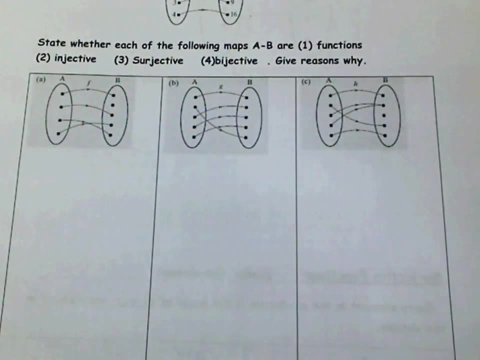 down here stay, whether each of the following maps, and mapping a to b, our function one functions are two injective functions, three surjective functions and four bijective functions, and give a reason for your answer. okay, so deal with each one separately. okay, so a graph number one, the first thing you're asked. 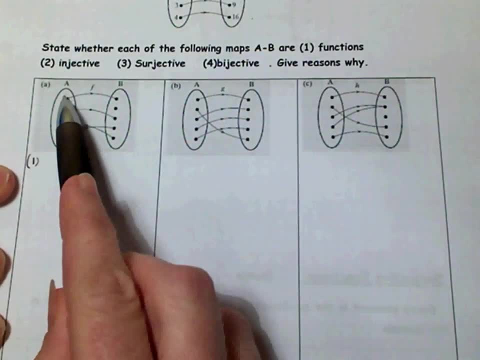 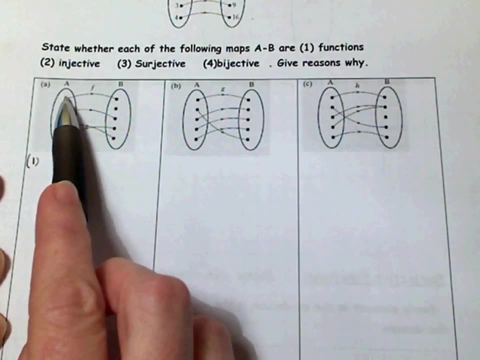 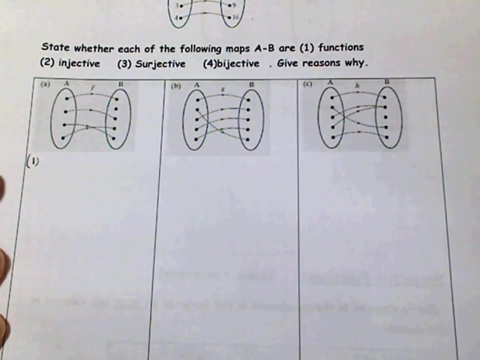 is. you're asked: is it a function? okay, so does every input and just have one output. okay, so is there another way to describe this? is in a, is there only one arrow going from? and each element in a? and yes, there is okay, so, and it's a function. 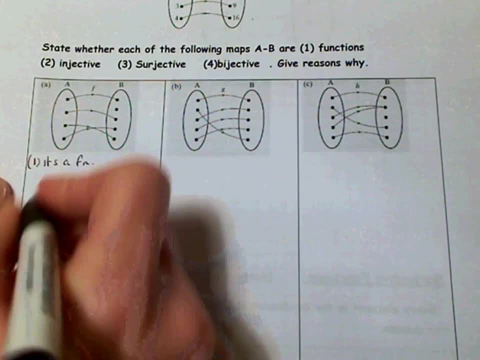 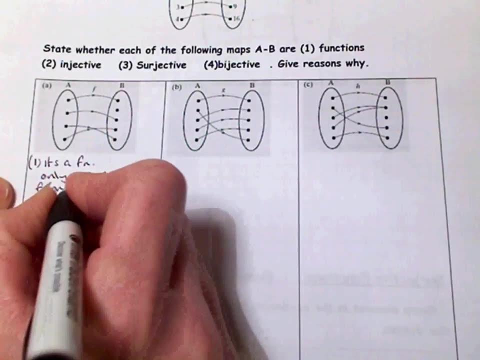 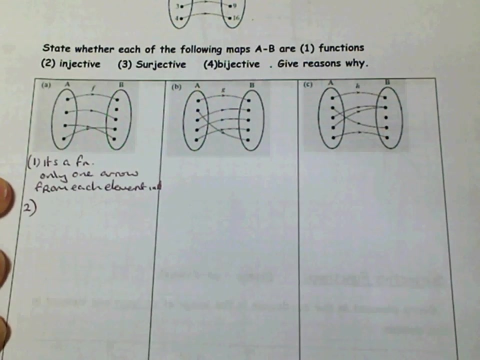 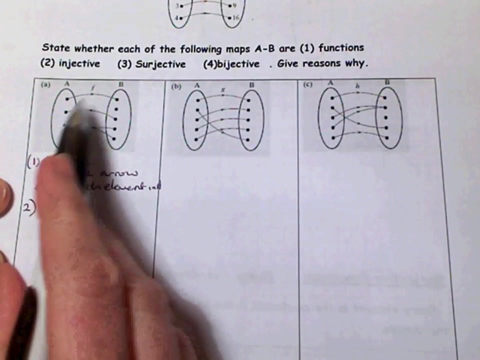 I'm just going to call the function fn. okay, and only one arrow from each element in a okay to. is it injective? so for every input is there a unique? I put: and yes, there is. it marks only on to one element in B. okay, so yes, and it's. 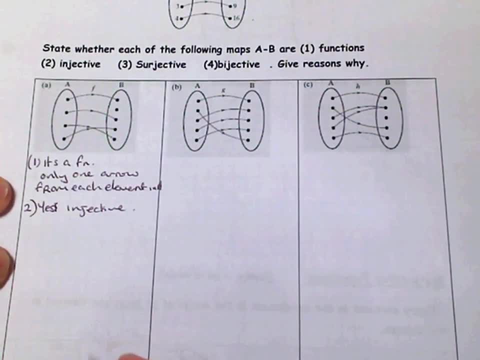 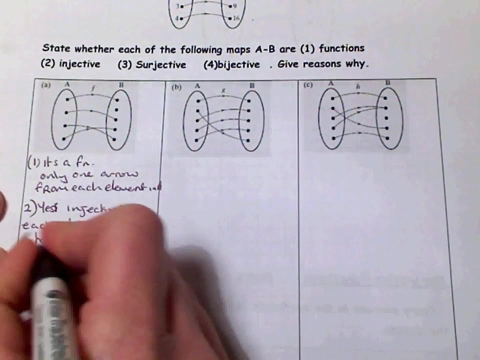 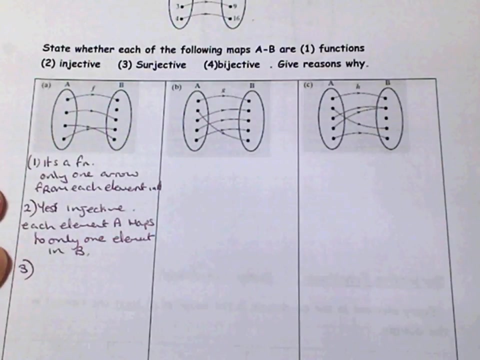 injective, okay, and the reason is that, and each element in a maps to only one element in B. okay, so only to one element in B, so maps to only one element in B. now the third thing we're asked is: is it surjective? okay, so first surjective and 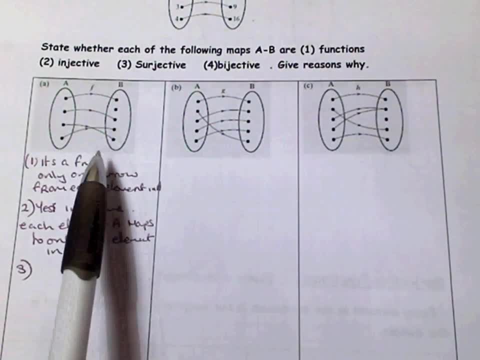 all of the elements of the co-domain have to be used. okay, so the range in the co-domain and have to be the same and the range in the co-domain in this and part a are not the same, because that's the range, that's the range, that's the. 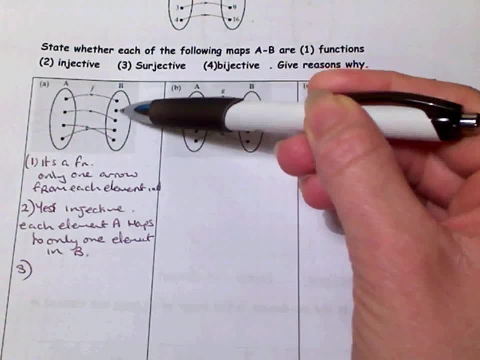 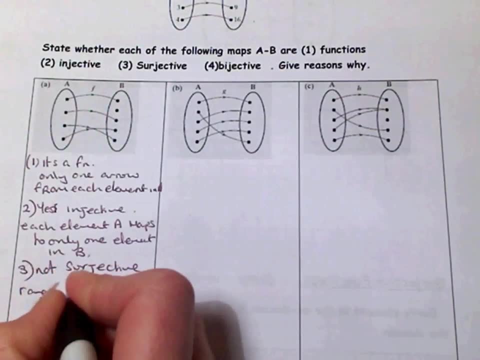 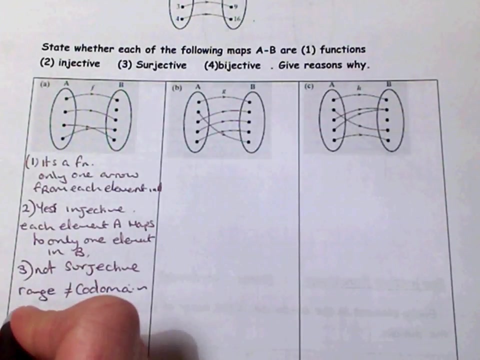 range, and that's the range where the lines connect. and this one isn't used. okay, so it's not surjective. okay, because the range is not equal to the co-domain. okay, and you can also say that all elements of the co-domain are not used. and the last one we're asked is: 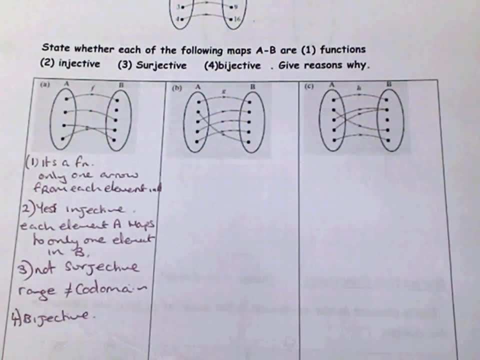 for a bijective: okay. so is this particular function bijective? and the answer is no, okay, so it's not bijective. okay, and the reason for that is because it's not injective. okay, and the reason for that is because it's not injective. it's not injective and surjective. remember to be bijective: the function. 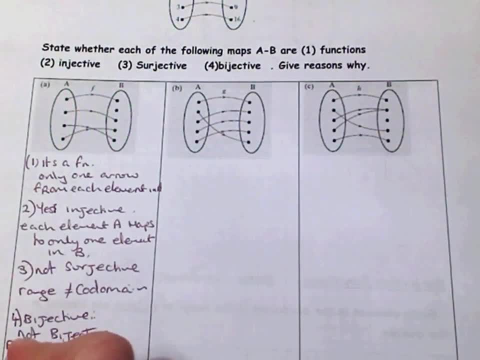 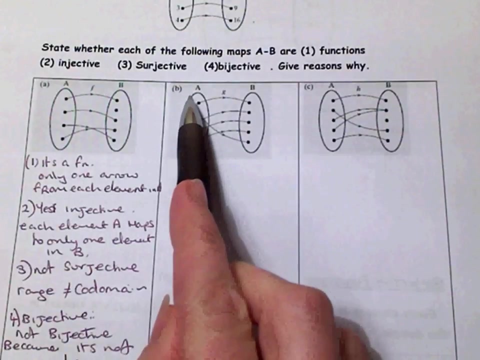 must be injective and surjective. so, and because it's not injective and surjective, okay now. so, moving on to part B, so you're given this function here and you're given the domain and the range in the co-domain over here. okay, so, first of, all. is it a function? yes, it is a function because. and the range in the co-domain over here: okay. so first of all, is it a function? yes, it is a function because. and the range in the co-domain over here: okay. so first of all, is it a function? yes, it is a function because. 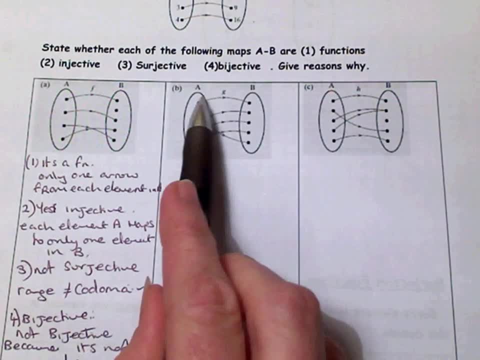 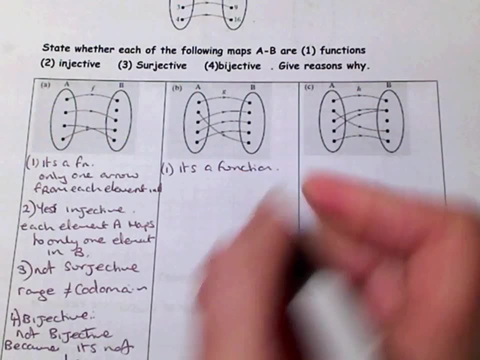 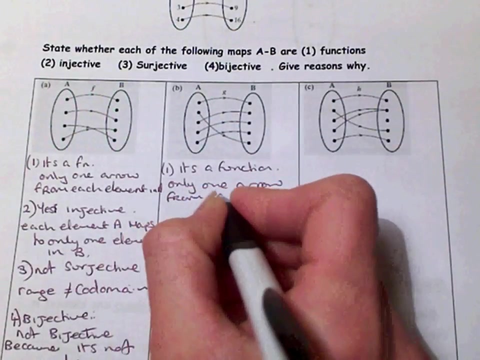 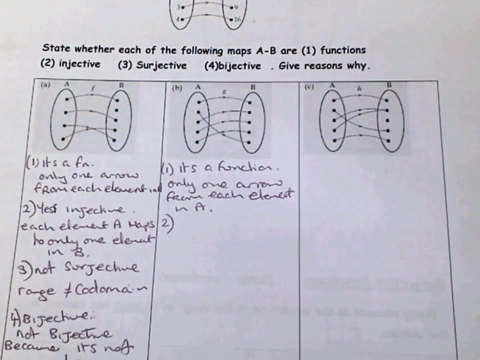 and each impulse only has one, one arrow going for it. so part one is: it's a function, okay, and once again, it's only one arrow from each element in a that's important to. is it injective? so does it? does each impulse have? and a unique. 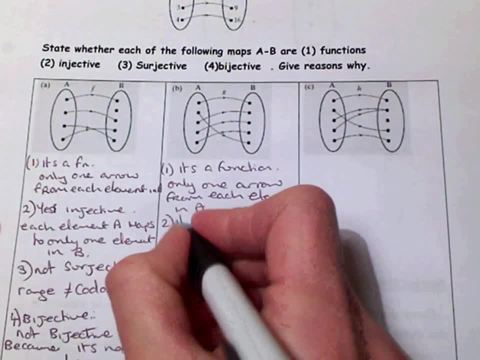 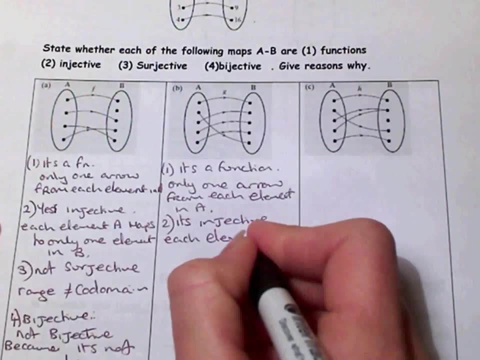 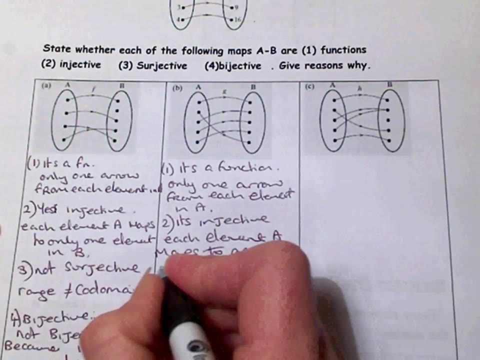 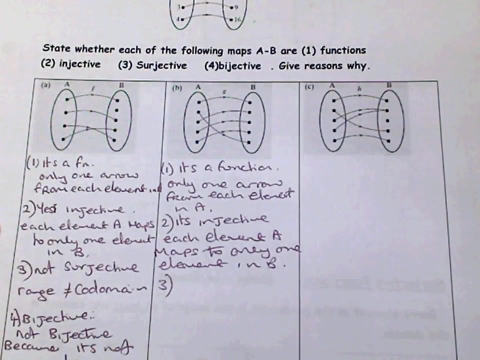 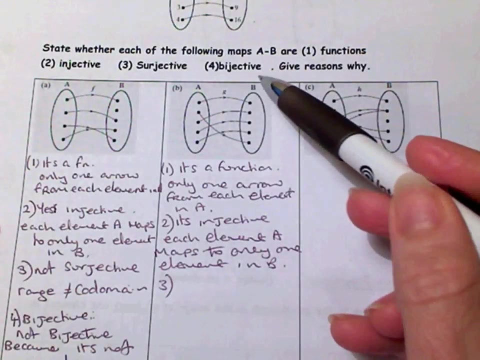 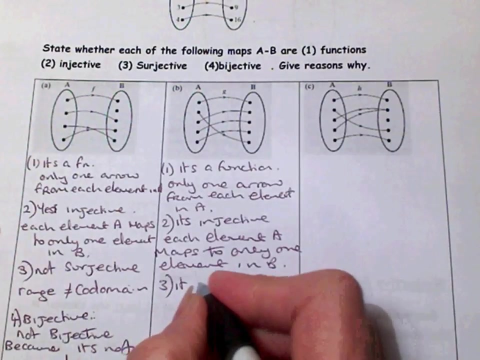 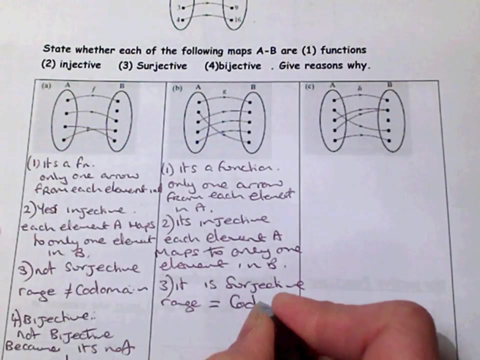 iPod? okay, yes, it does so. and it's injective. okay, so each element, and in a maps to only one element in B, so a unique. I post Three. is it surjective? Okay, so with surjective, remember the range and the co-domain must be equal. Okay, So it is surjective. so it is surjective, Okay, and you can say that the range is equal to the co-domain. Okay, 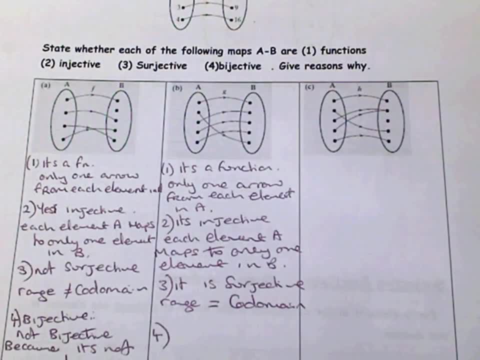 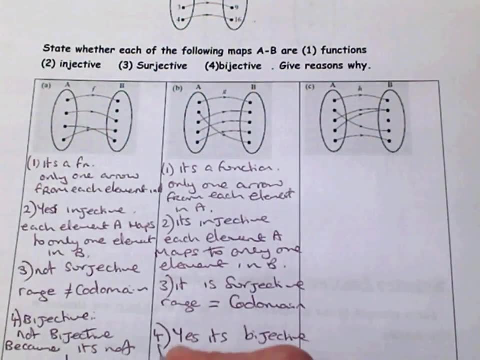 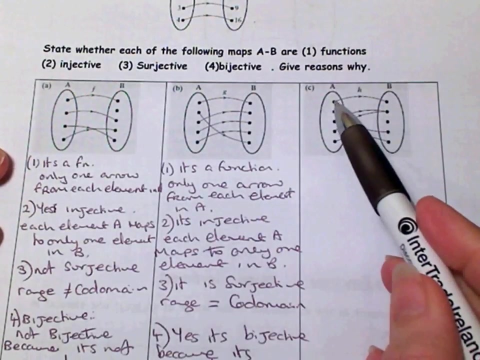 And number four: is it bijective? And yes, it is bijective. So, yes, it's bijective, because it's injective and surjective. Okay, And part C over here, Okay. So we're asked: is it a function? first of all, So we follow the lines across, So only one line coming from each of the two. 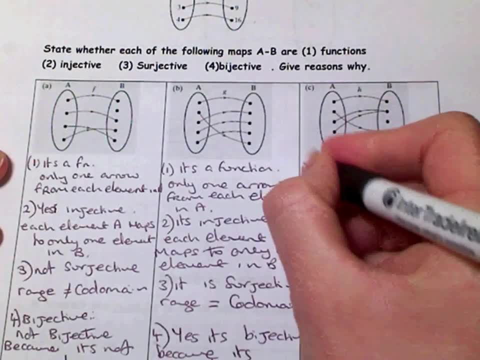 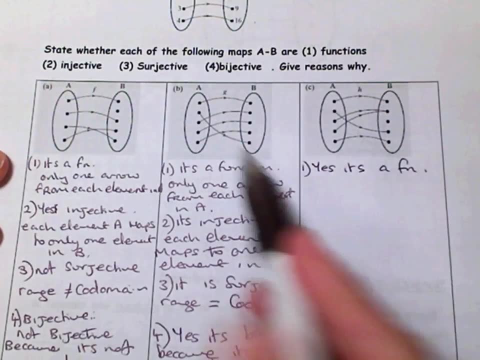 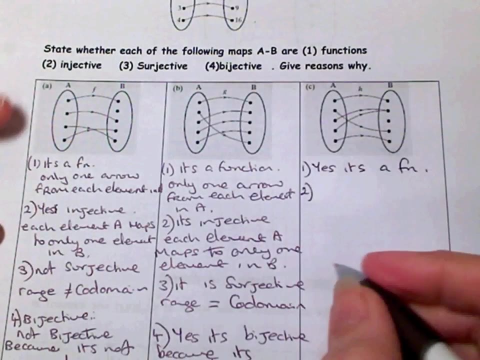 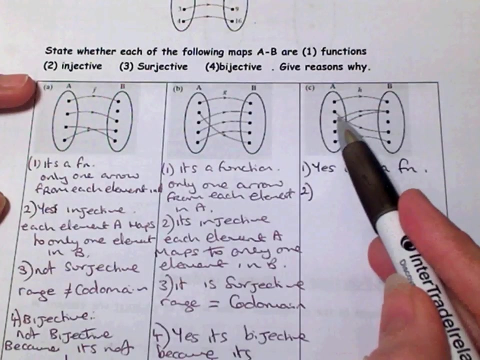 Of our elements in A. So part one, there is: yes, it's a function. So yes, it's a function, Okay, And the same reason as the others, because only one line going from each of the elements in A. Number two, is it injective. So for each input is there a unique output, Okay, And you can see there that these 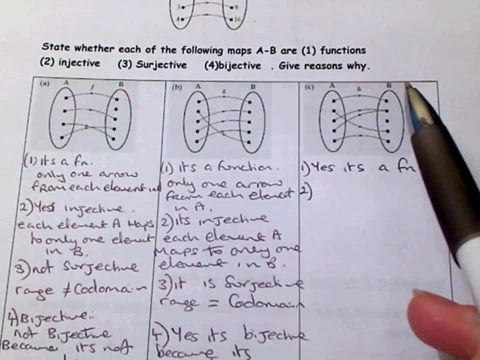 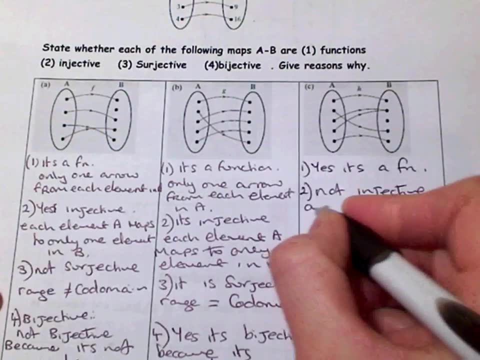 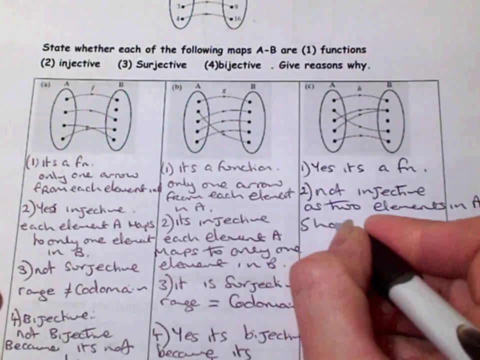 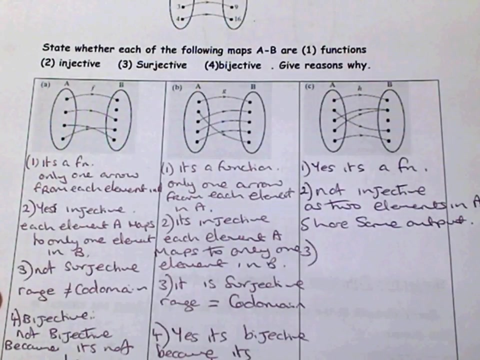 two elements here, share the one I put, so it's not a unique. I put so, therefore, and it's not injective as em. two elements in a share the same I push, so it's not unique. number three: is it surjective? okay, so if you look here, surjective, okay. 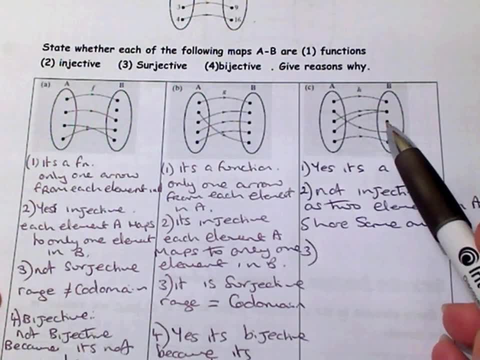 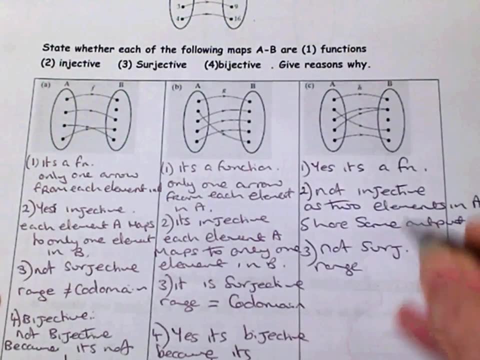 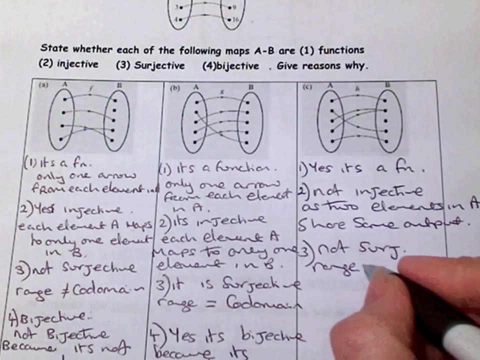 so looking, okay, except for this one here. okay so, and the range. so it's not surjective, because the range over here, remember the range is this one, this one, this one and this one, and it's not equal to the co-domain because one of the elements isn't used, so it's not equal to the co-domain. 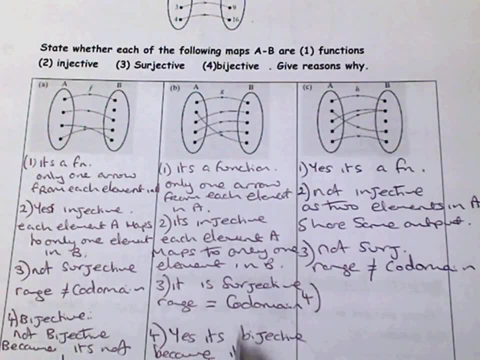 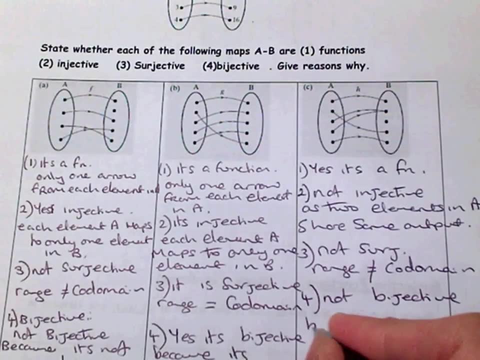 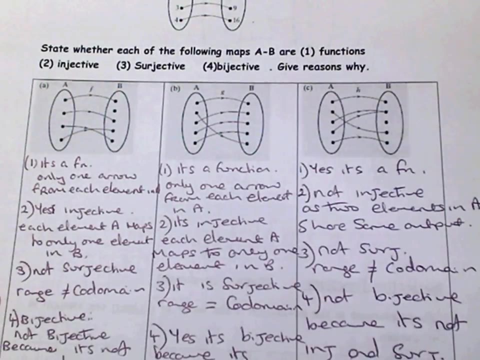 okay. and number four is: we're asked: is it bijective? then it can't be bijective. so it's not bijective, okay, because, and it's not not injective and surjective okay. that's a very important example, as you will see when you go on into the. 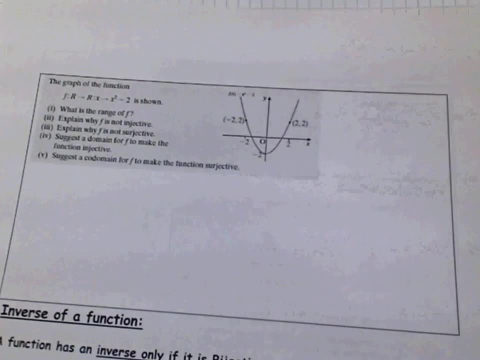 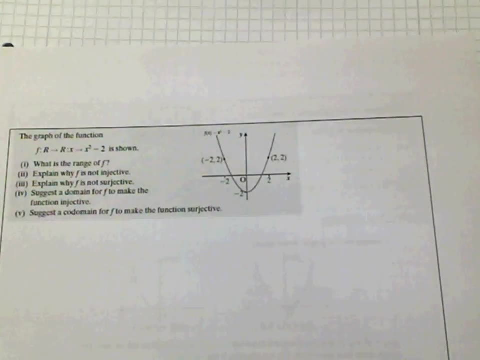 exercise. okay, so one more example that I want to look at is this one here on the graph. okay, so one more example that I want to look at is this one here on the graph of the function. okay, so you're given the graph and you're asked some questions. 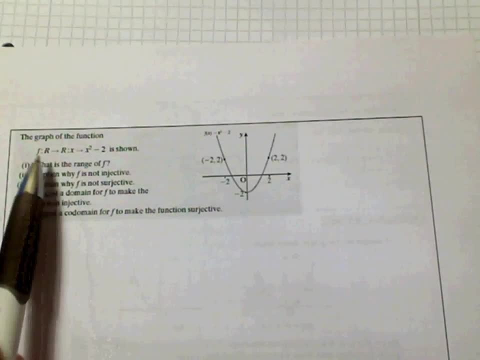 on the graph. okay, so you're given the function and you're told that the domain is real numbers and that the co-domain is also real numbers. so you're asked for the range of the function. that's the first thing you're asked for. so when a 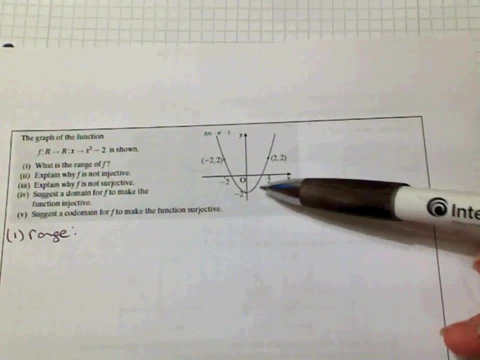 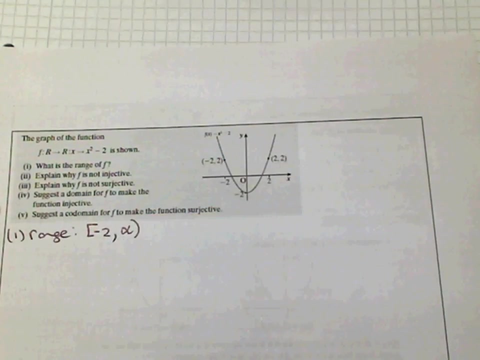 question like this, you have to look closely at the graph, okay, so the range of the function, remember, the range is the output, so it's the y-value. so we're looking at the y values and it's definitely starts with the value of the at minus two, so we have minus two, but it goes on and on, so it goes to infinity and we have our. 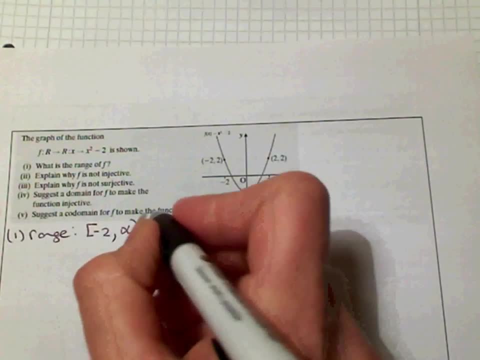 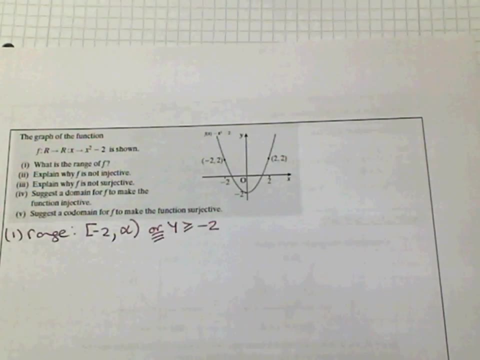 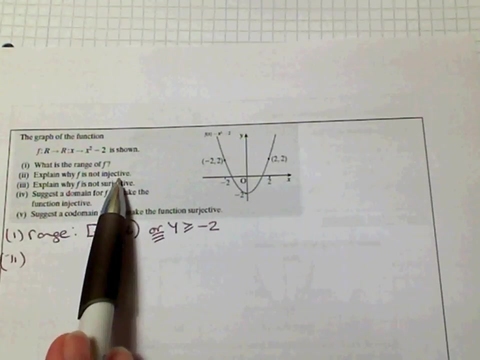 curved bracket. okay, you could also write that, as the y values are greater than or equal to minus two, they're the exact same thing that i've written there. okay, part two. you're asked: explain why f is not injective. okay, so for injective. um, you can look when you're given a graph always. 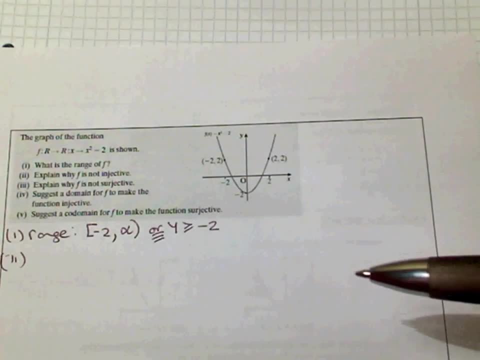 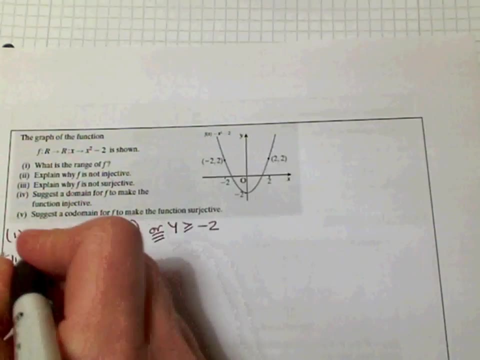 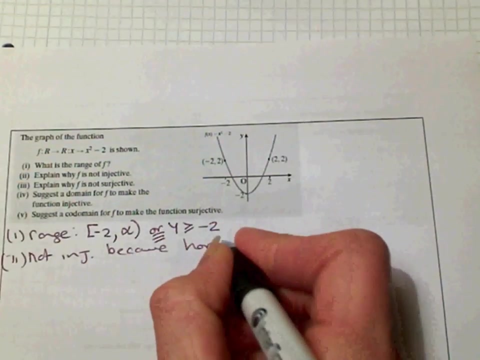 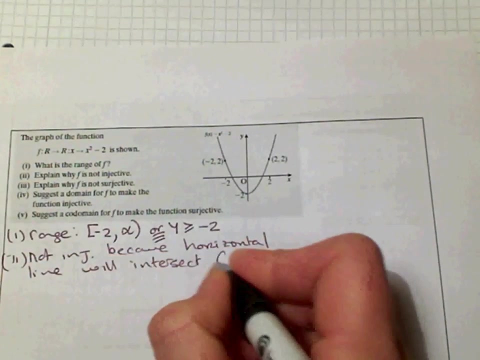 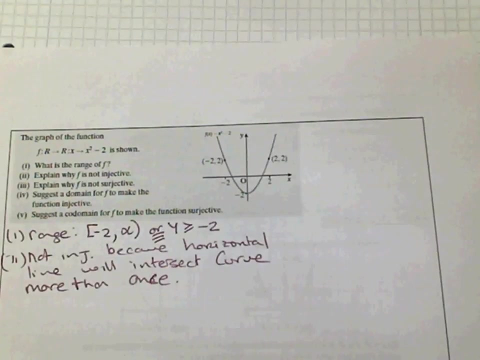 um, think first with this horizontal line test. okay, so, first of all, um, if you draw a horizontal line across here, it's going to intersect the graph twice. okay, so, um, it's not injective, uh, because horizontal line will intersect curve more than than once. um, okay, now there is another um reason for this, and the reason is that. 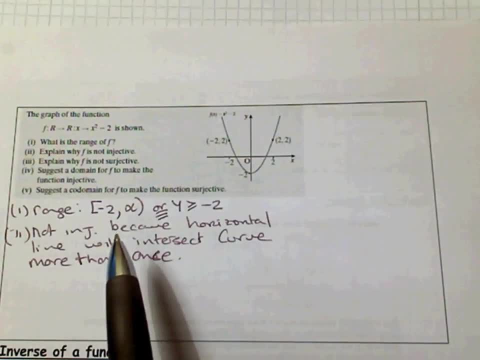 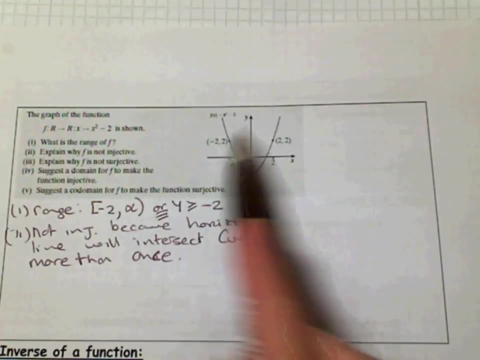 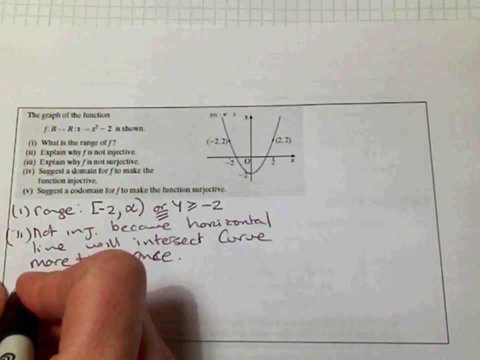 if you look, the definition of an injective function is that it has a unique. every input has a unique output. if you look here: if you input minus two, you get two. if you input two, you get two. okay, so, um, you can say that. um, also, another reason would be that minus two, uh gives. 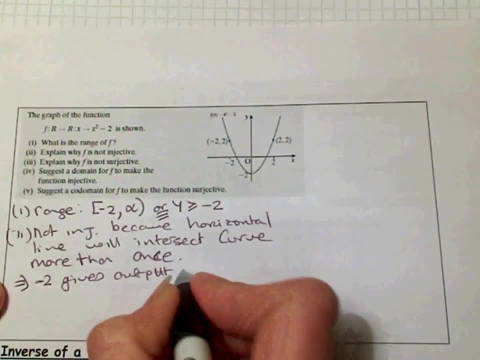 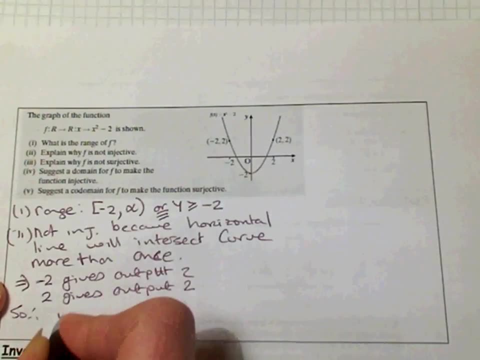 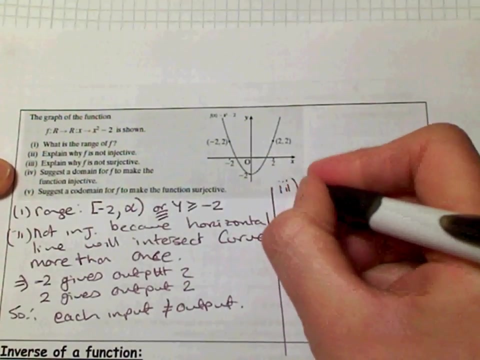 an an output of two, and two gives an output of two. so therefore each input does not have a unique output. okay, so that's just another reason for that. okay, part three: you're asked: explain why f is not surjective. okay, so remember. uh, the conditions of the input are not different. 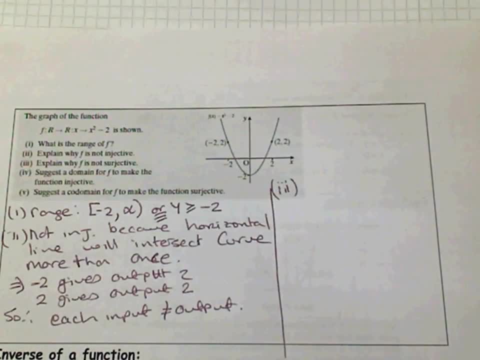 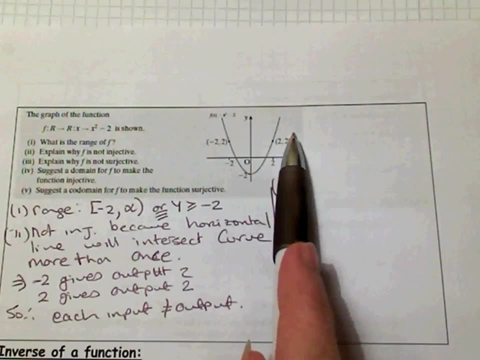 for surjective was that the horizontal line will intersect at least twice. okay, now you could fall into the trap here, because yes, it does intersect at least twice. okay, but one of the major conditions was that for a surjective function, the range must equal the co-domain. now we've already said that. 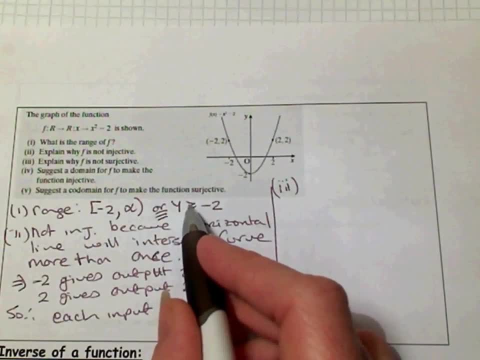 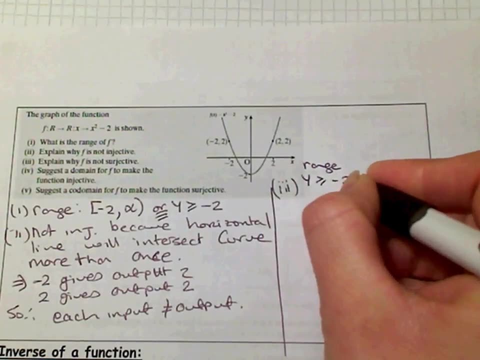 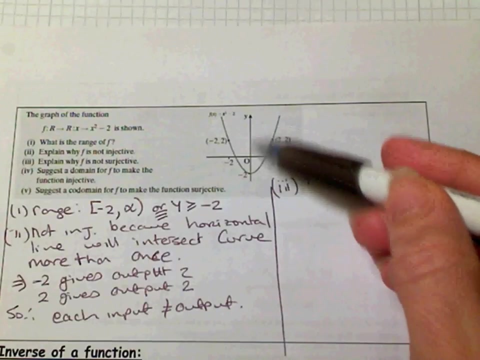 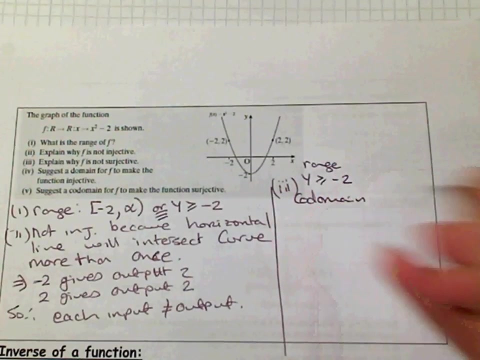 the range is values, and the range are values greater than or equal to minus two. remember that the range was greater than or equal to minus two. now, if you look at the co-domain, which is all the possible y values, okay, so the co-domain were the set of real numbers, so the co-domain were basically: 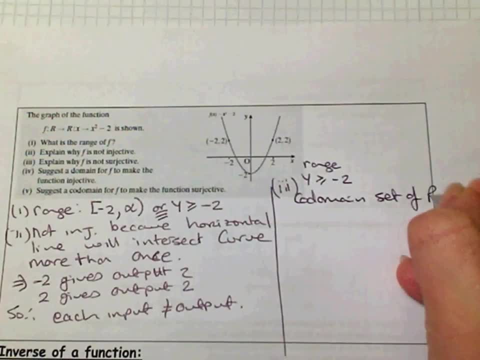 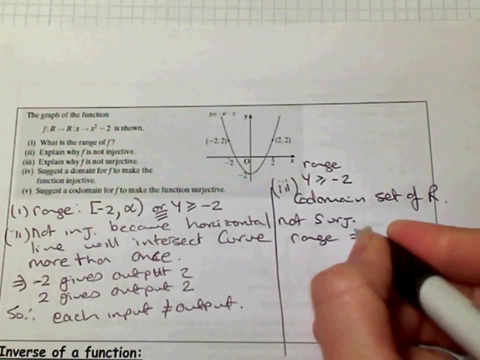 any y values, so the set of real numbers. okay. so therefore, the reason it's not surjective is because the range does not equal to the co range domain. so, as i pointed out at the start there, be careful that you don't fall into the trap when 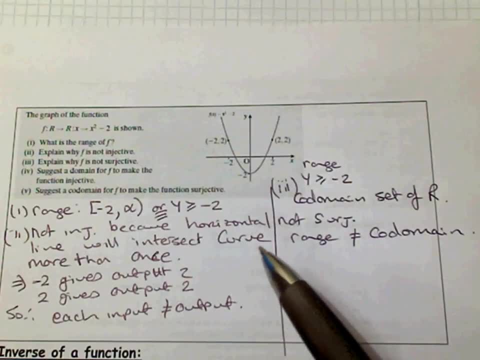 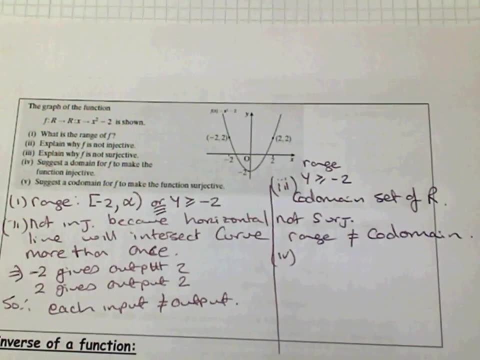 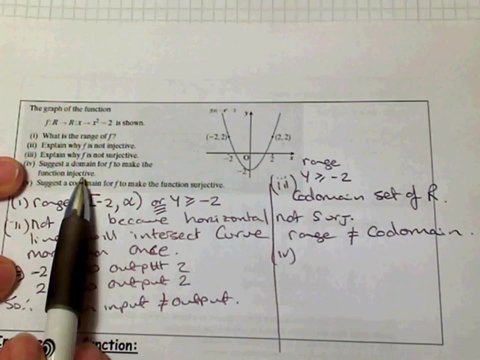 you're given the graph of just looking at the horizontal line, always look at the range and always look at the co-domain, part four- and suggest a domain for f. to make the function injective, so suggest a domain for x. and to make the function injective, so an injective function. 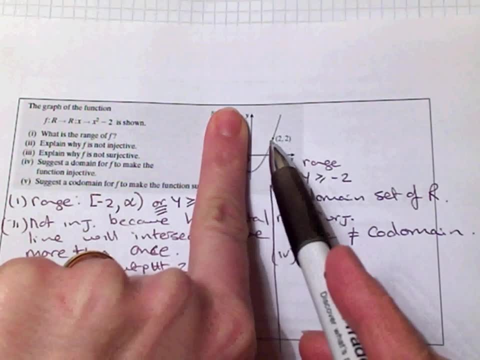 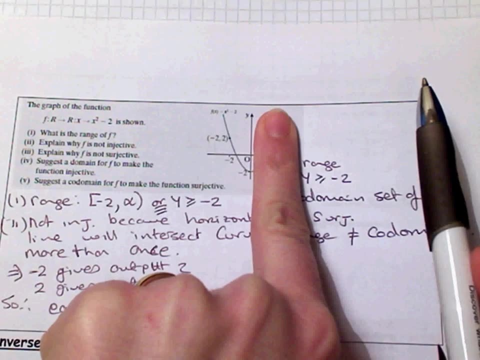 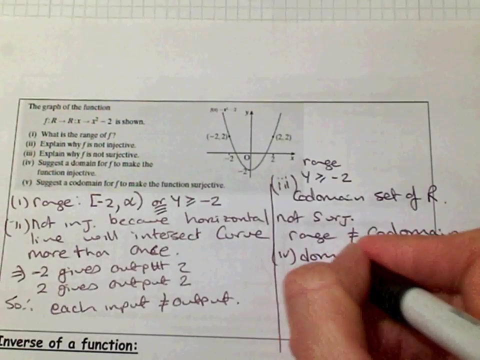 if you look at the graph here and the horizontal line, if i were to cut off that side, the horizontal line would intersect just once, okay. or to do the opposite, to cut off this side, the horizontal line would intersect just once. so therefore, i could talk about a domain where the x values are just greater than or equal to zero, or 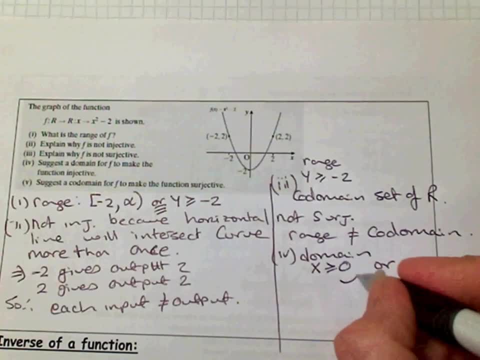 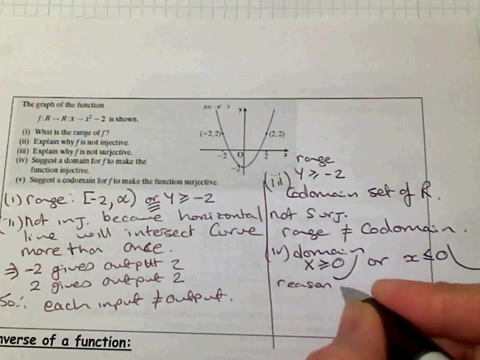 and that would give me greater than or equal to zero. give me a curve looking like that. or I could say less than or equal to zero, which would give me a curve looking like that. okay, And either of those is the correct answer, and the reason would be- I know you're not asked for it. 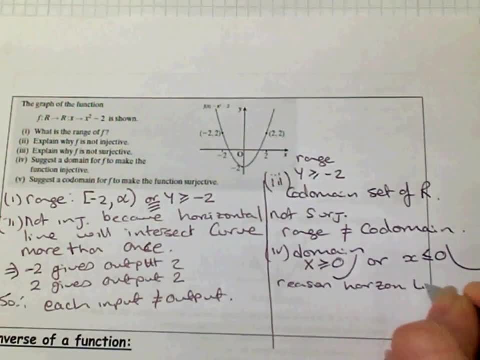 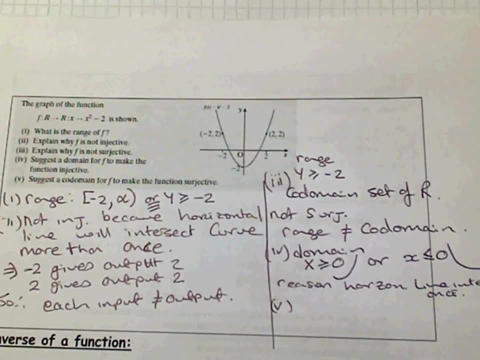 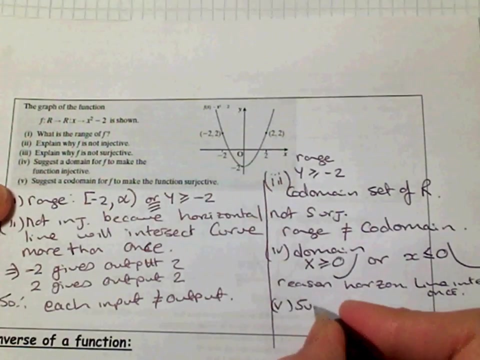 but the reason is that the horizontal line will intersect once. okay. And part five: suggest a codomain for f to make the function surjective. So suggest a codomain for f to make the function surjective. okay, So remember that to be surjective, the range must equal the codomain. 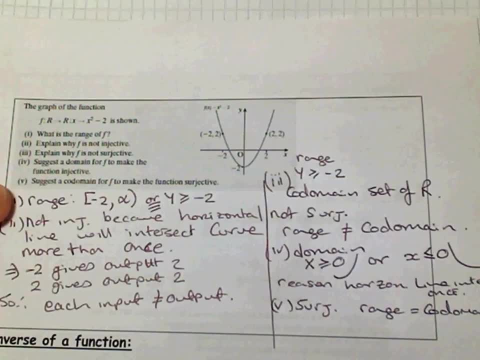 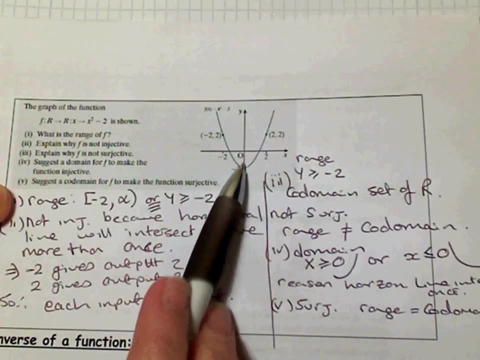 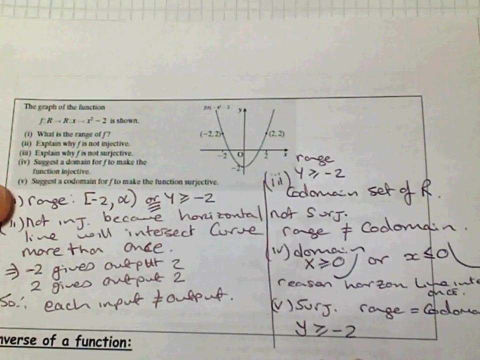 And I said that the codomain was the set of real numbers. okay, So if you restrict the codomain to just one y values greater than or equal to minus two, then you end up having the range equal to the codomain, okay. So therefore it would be a surjective function.